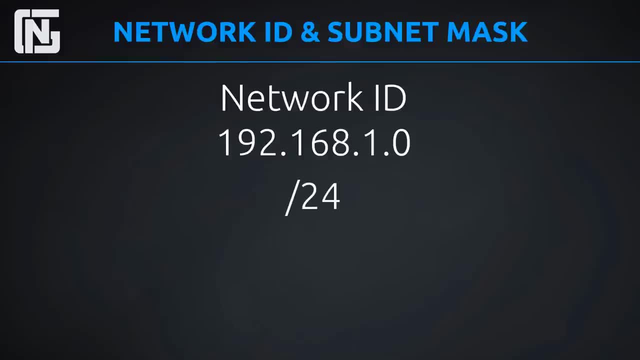 is All right. so the slash 24 is called the CIDR notation, or CIDR notation, which means Classless Inter-Domain Routing. Just remember that this is called the CIDR notation and normally you'll see it like this: you'll see it like 192.168.1.0, slash 24, and 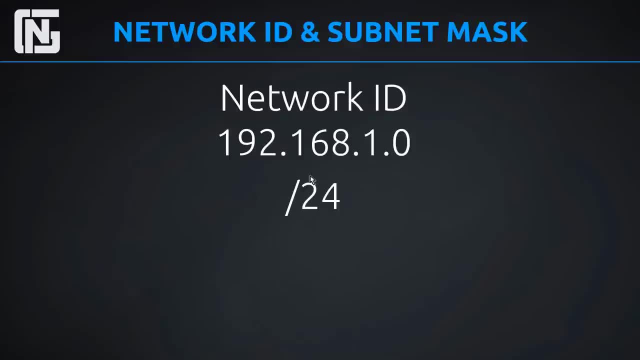 this is called the CIDR notation, and if you're using the CIDR notation, you're going to need the. What this means is this is telling you how many binary digits are turned on in the subnet mask. Let's look at that: 24 binary digits. Our subnet mask is something that's written in addition to. 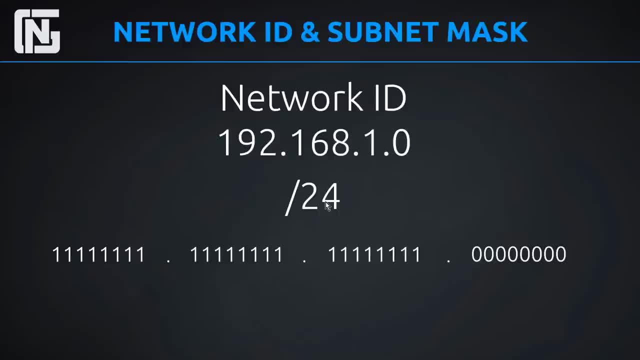 our network ID or our IP address. You've heard this before: It's 192.168.1.5 with a subnet mask of 255.255.255.0, right, So that is what we're referring to here. Now again the CIDR notation. 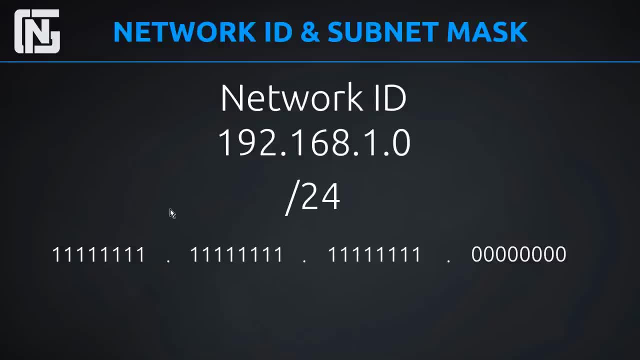 slash 24 refers to the number of bits in the subnet mask. So here we're looking at the subnet mask- actually We're looking at it in binary only for now- And we can see that the first 24 bits are all turned on. So that's 8 plus 8 is 16 plus another 8 is 24.. So the first 24 bits are all. 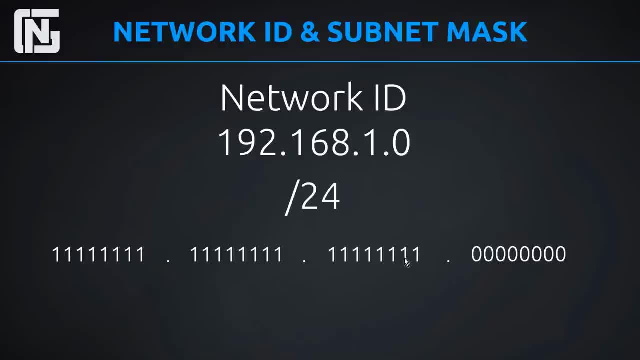 turned on And if we translate this, we're going to see that the first 24 bits are all turned on. If we translate this from decimal to binary, it'll give us 255.255.255.0.. And we could use our 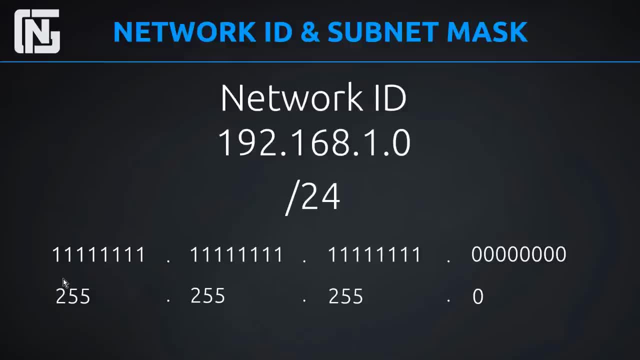 great, awesome chart for doing that, But I figured this one was simple enough. We didn't really need it. Remember we already talked about: if you have all ones in an octet, that always equals 255.. So you can remember that, guys. So 255.255.255.0 is actually our subnet mask And we know this just. 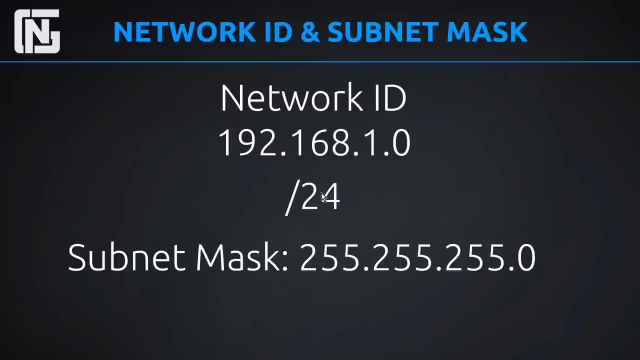 by looking at the SIDR notation. We know this just by looking at the CIDR. If the CIDR is slash 24, we know our mask is 255.255.255.0.. And if we know our mask is 255.255.255.0, we know our. 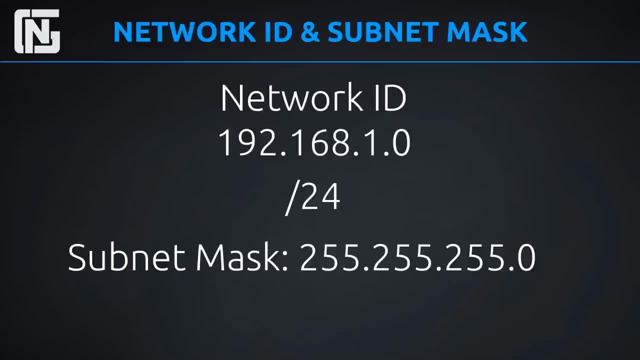 CIDR is slash 24.. So that's how those two are related, guys. They're both masks, All right. So now we're going to figure out what the mask actually means a little more whenever we're determining what our network ID is. So let's look at an example on that. Here we're changing it up. 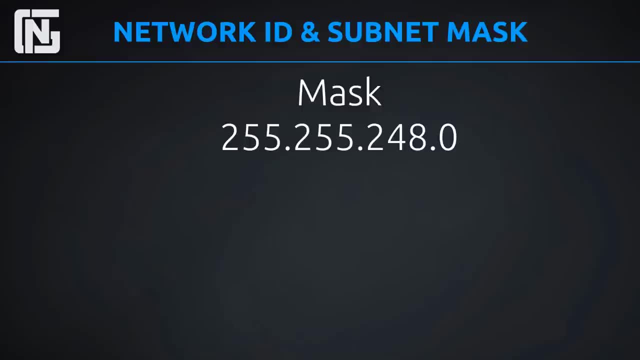 a bit. We're just showing the mask at the top of the screen And here we have 255.255.248.0.. We're going to go ahead and bring up our nice chart here for reference And we can figure out actually our CIDR notation from the mask directly, Remember. 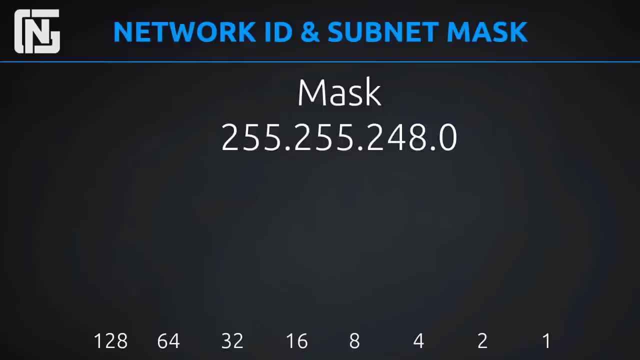 we said, if we knew the mask was 255.255.255.0,, we knew it was a slash 24 CIDR. Well, in this case we have the mask 255.255.248.0.. So let's figure out what our CIDR is there And how we do that is. 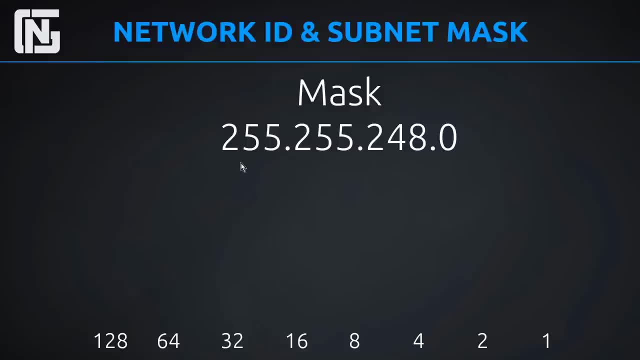 255.255.255 is all ones, So these are all ones in the subnet mask here, But 248 is not. We know it right, We know it's not. And then 0 is all 0s And the fourth octet is just all 0s, But 248 is the. 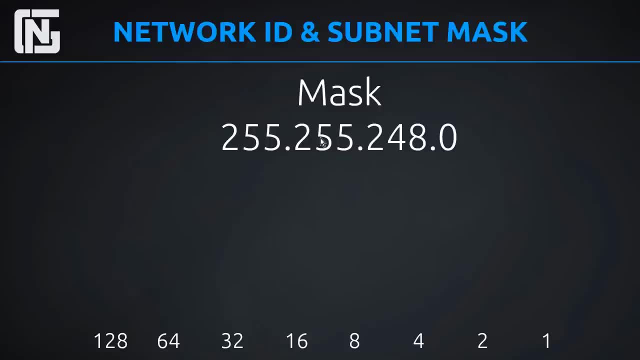 one. we've got to figure out how many bits there are, Because we know that there's 8 bits here and there's 8 bits here, So that's 16.. So in this third octet we're going to be adding from 16 up. 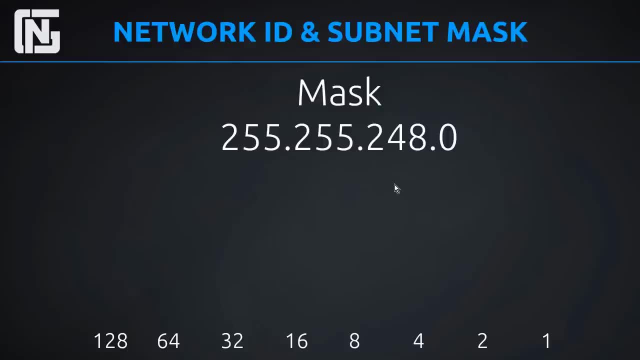 until we get to 248 in decimal format, which will give us our CIDR notation. All right. So here's how that works, guys. We have 255.255, and then 128 plus 64, which is 192.. Not there yet? 192 plus. 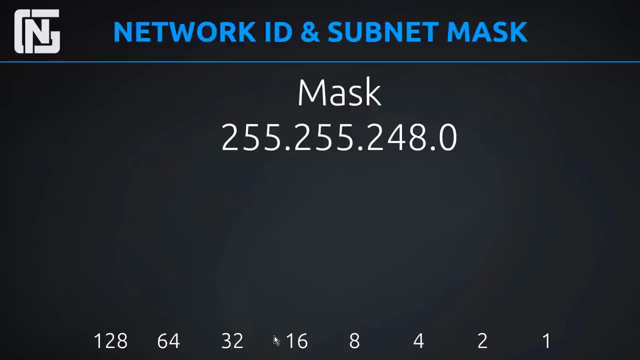 32,, which is 224.. Not there yet. 224 plus 16,, which is 240.. Not there yet. 240 plus 8 is 248.. Hey, there we are. So we know these are our subnetting bits And everything else is considered to be a. 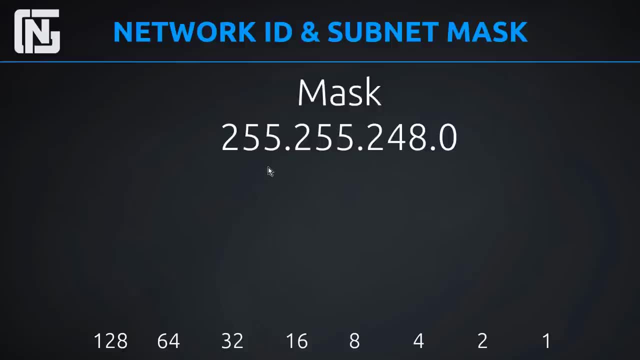 host bit, All right. So what does that mean for our CIDR? Well, we knew we had 255.255, and that was 8 plus 8 was 16.. So we're going to add a slash 16.. And then we add slash 16 plus. 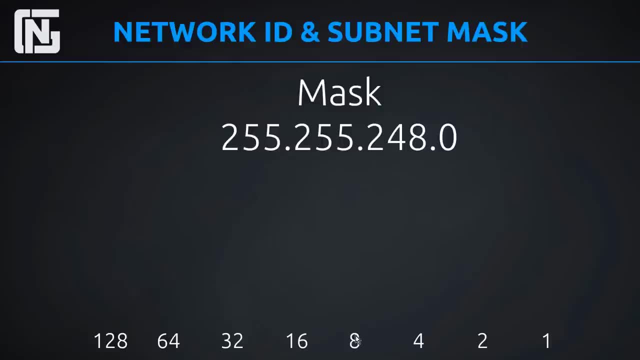 17,, 18,, 19,, 20,, 21,. right, So that's how many bits are in our subnet mask? There's 21 bits in our mask, giving us our CIDR of slash 21.. That's how we get that guys from the mask. All right, So? 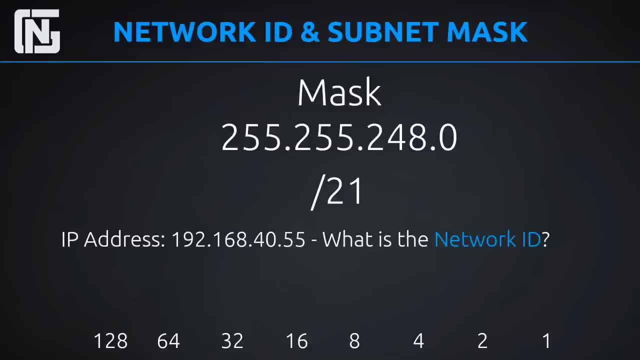 now that we know that, let's go ahead and look at an IP address. Here we have an IP address 192.168.40.55.. So what the heck is a network? Well, we're given the mask and we're given the slash 21.. And from that we can figure out what. 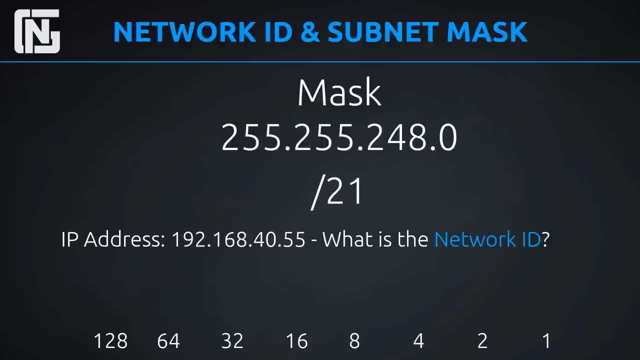 the actual network ID is. It's not always as simple as it may seem, So let's look at an example here. We can start off by knowing that 192 and 168 are going to be a part of the network ID, because the mask includes all ones there, And if there's all ones, that means you need to use. 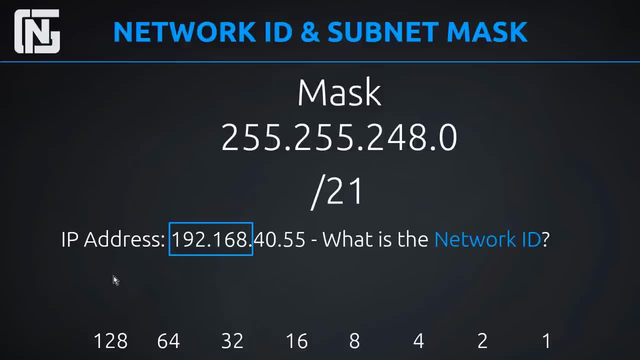 these numbers right. In fact, the mask means use all the numbers. wherever the mask has a one, All right, And we'll see that here coming shortly. So if our first two octets in our mask have 255 and 255, then we know we need to use the first two octets of our IP address in. 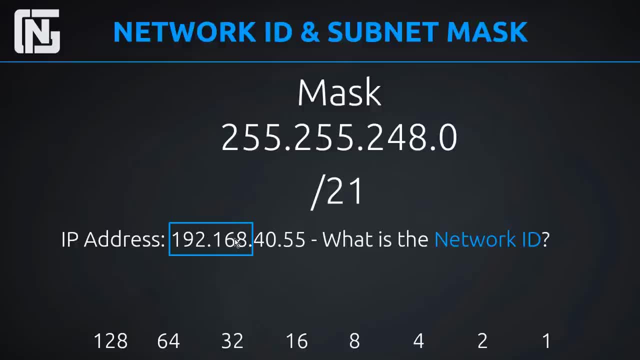 the network ID. So it's going to start with 192.168.. Here, where it gets a little bit more fuzzy is we go into the third octet, because that's where the mask is a little bit fuzzy as well. That's where our 21 bits go into. So we're at 16, then they bleed into the third octet until. 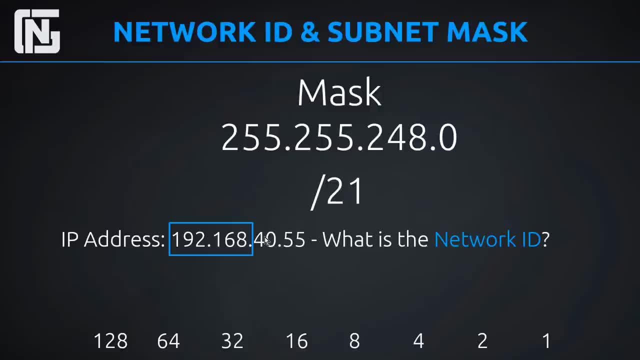 the 21st bit, And then our mask cuts off somewhere in that third octet. So let's look at this a little more closely. That third octet is actually comprised of the following binary digits: It's actually 40, right? And we could easily determine that by saying: oh, 40 is 32 plus 8.. 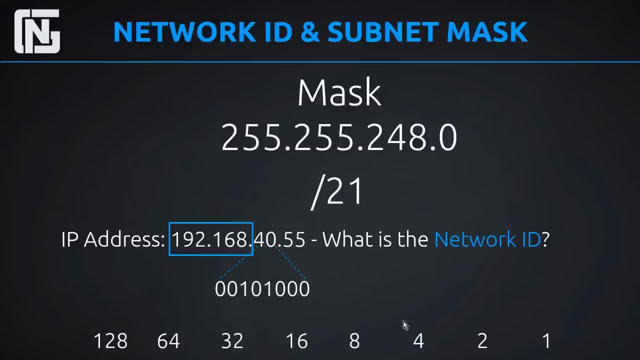 So these would be turned on, So it's 00101000.. That's how we got that there, Super easy, As long as you have your super cool chart there. that I said I wasn't going to give a name, but I ended. 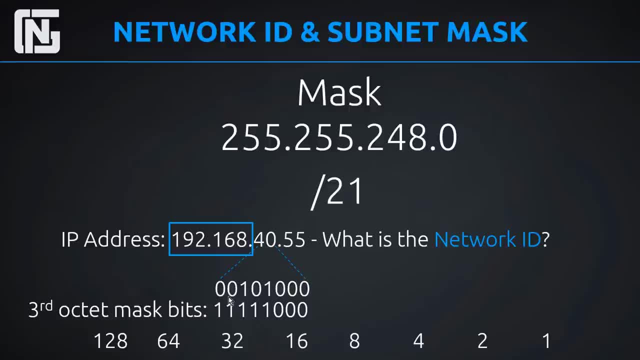 up giving it multiple names. All right. So here we are. We're looking at the third octet, and the rest of them are 1111100.. And how did we calculate that? We said 128 plus 64 plus 32 plus. 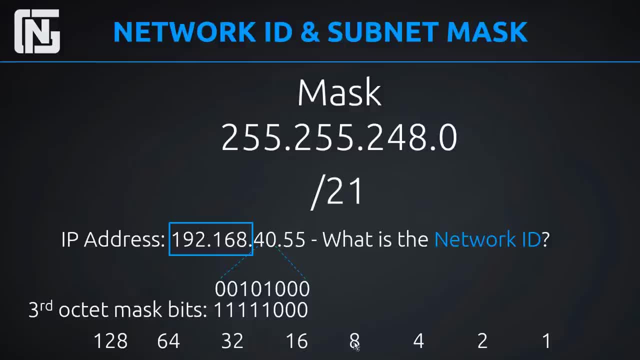 16 plus 8 added up to 248.. So that's how we knew it was 11111.. And the rest of them were zeros. So when we put the mask up against our IP address here, we can see that everything here where we 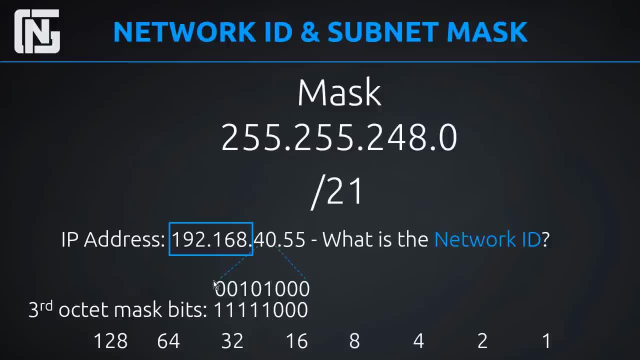 have our mask. all these bits in the IP address need to be used. So we're going to go into the third octet, put our mask on and we're going to pick the IP address. So we're going to put our in the network id, because the subnet mask tells us what our network id is, or our subnet id, subnet. 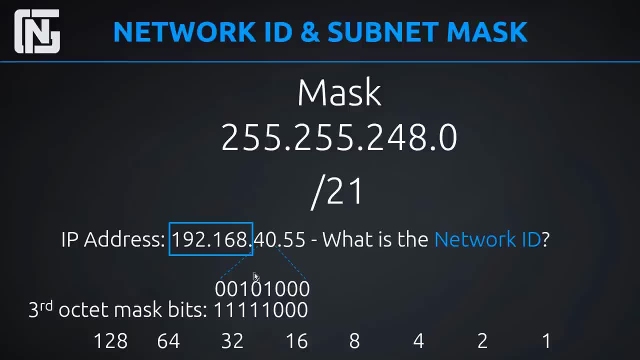 mask, network mask, subnet id, network id- they're all generally the same term. anyhow, these digits in the mask in our in our third octet, are telling us that 40 is also part of our network id, because the bits that go along with the extension of the subnet mask here include 40 in them. 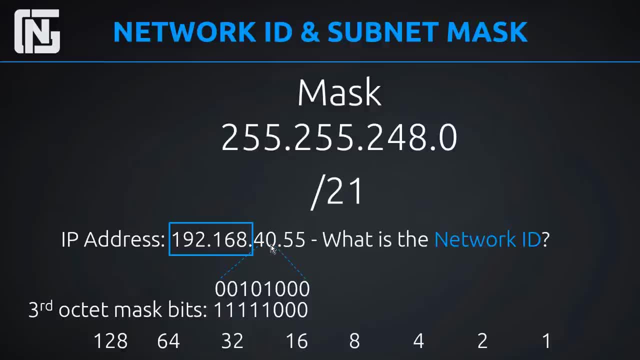 now, if our ip address given was 192.168.41.55, then 41 wouldn't actually be part of our ip or part of our network id. it would still be 40 because our mask said: only use these bits here in the mask. all right, we're going to do a few of these, so don't worry. now let's go ahead and look. 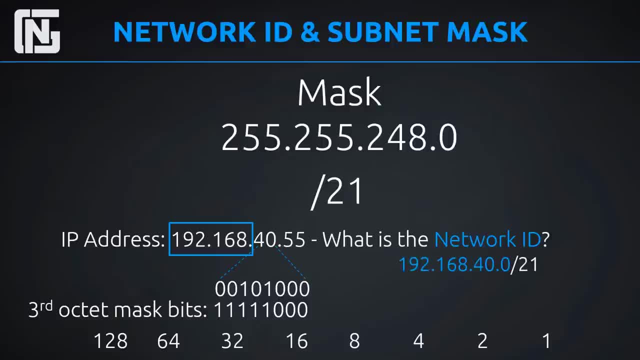 at what that actually means. that means that our network id is 192.168.40.0 and we've written it here in sitter notation and we're going to do a few of these, so don't worry. now let's go ahead and look at what that actually means and what this means, and we've written the network id. 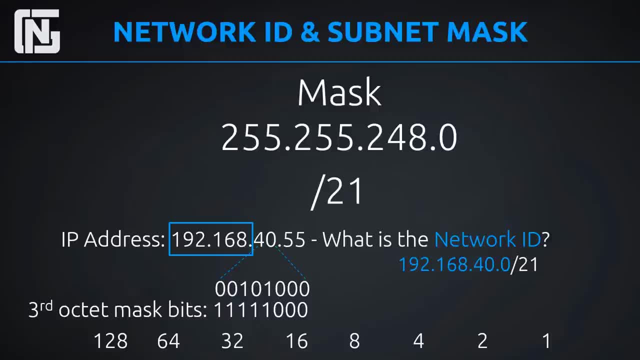 notation- cidr notation- by putting the slash 21 at the end. and we also know that our subnet mask is 255.255.2480. and i've written all these here together because generally that's what you'll do, or generally that's what i do. i write the network id plus the cidr notation plus the subnet mask. 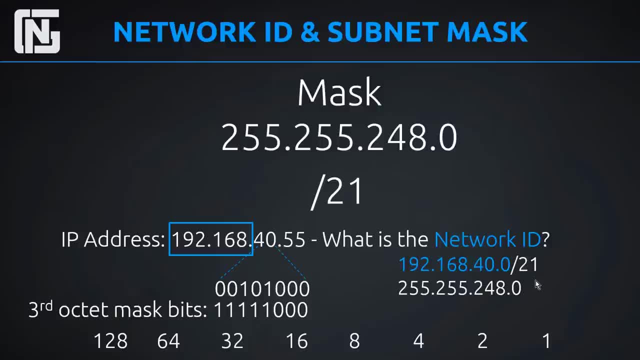 sometimes i'll just use the cidr. depends on who's looking at my documentation. right, some people don't know what the cidr is, but that's how we use our mask to determine what our network id is. so our network id is 192.168.40.0, and we're going to write the network id plus the cidr notation, plus the. 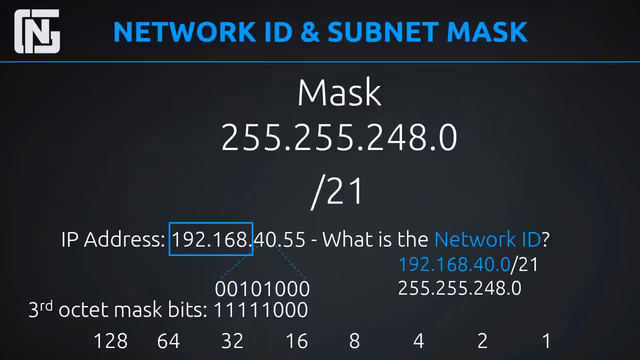 to 168, 40.0 guys 40.0, and that includes a lot of hosts. these are all host bits here. so we actually have the entire fourth octet and we also have three bits of the third octet are all host bits. so 41.55 is even a host, but i'm not going to get into that. that's where it can start getting a. 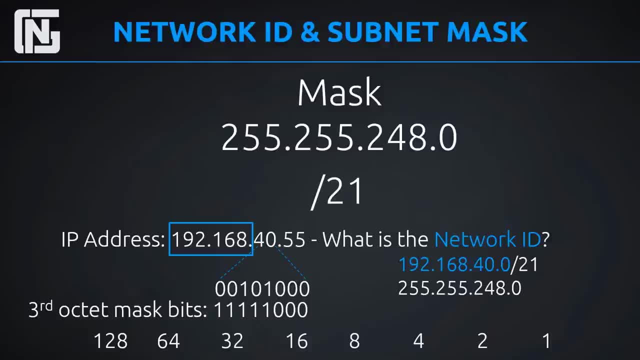 little more confusing. for now, let's just understand how we can take our mask and figure out what the network id is. really dump everything else out of your brain, just just understand this. how do we take our mask and our cidr and figure out what our network id is? given an ip address, that's what we 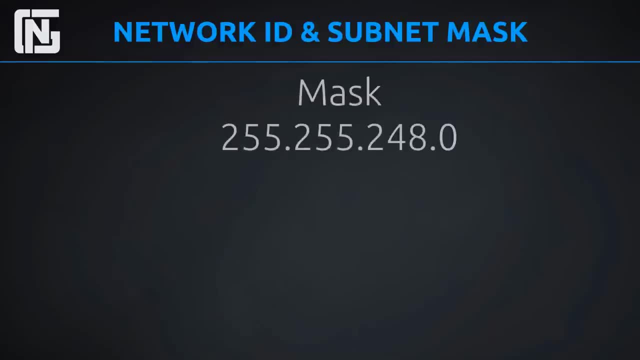 need to be focusing on right at this moment. so let's look at another example. here we have the same exact mask and we have our sweet super cool chart. then we have our cidr notation, and this is all the same as the last exercise. so you know how we figured that out. now we have a slightly 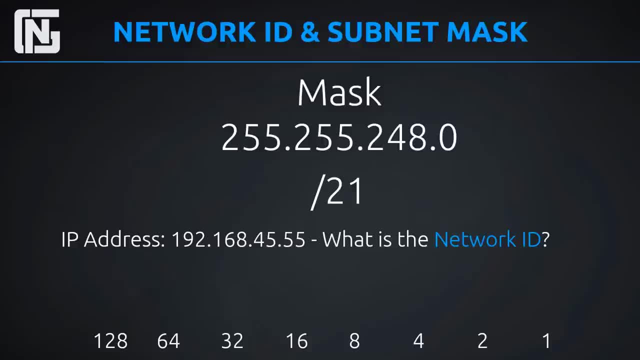 different ip address. it's 192.168.45.55. so what is the network id? well, we know again that 192 and 168 will be used in the network id because we have all 255s in the mask portion of those two octets right. so now we need 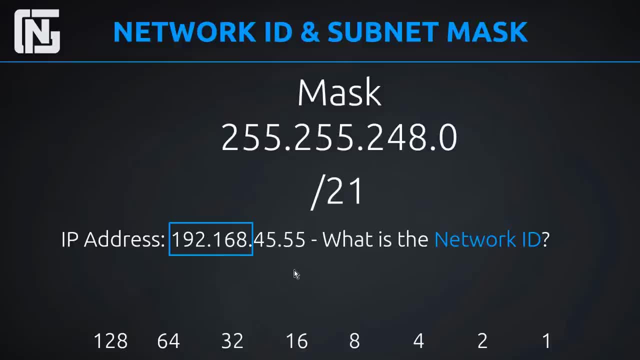 to look into the third octet here and we need to break out it, break it out into binary. when we break it down into binary we see it's zero, zero, one, zero one, one, zero one. and then when we put that up against the mask in the third octet, 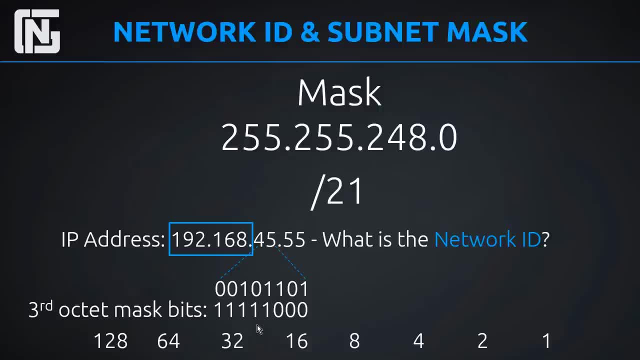 we see that these are the only numbers that should match right here. these other bits are actually host bits. they don't have anything to do with the network id. only the masks can tell us exactly which bits to use in our network id. so far they've told us 192.168, and now they've told us also: 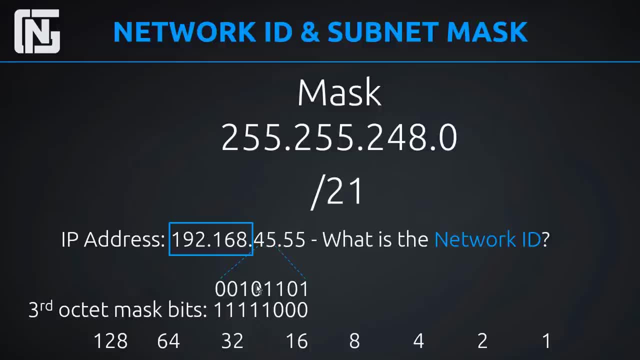 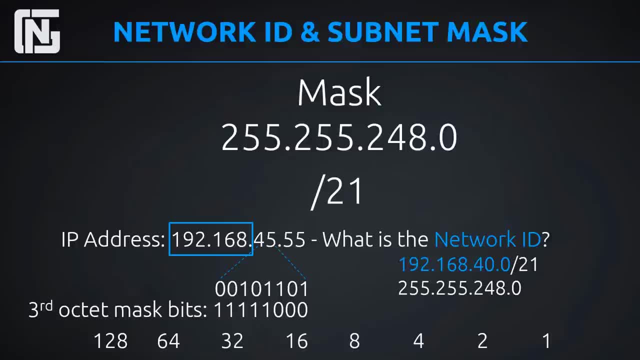 addresses like this. however, guys, be confident and know that whenever you look at things in binary and you learn it this way, it's so much easier to understand in the long run. that's why we're jumping into some more relatively complicated things right off the bat. so it's a good thing. 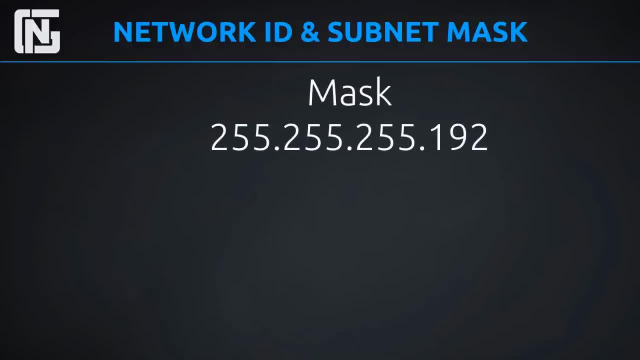 all right, let's look at another example. here we have a new mask all the way into the fourth octet: two, five, five, dot two, five, five, dot, two, five, five, dot one ninety two. so let's go ahead and think here, and actually let's think without using our chart, let's just 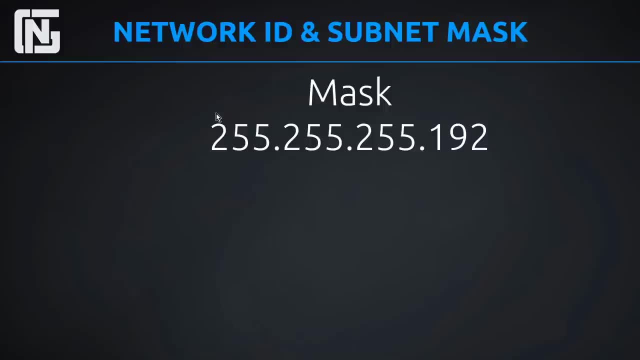 think, what could the cidr notation be? well, we know that two, five, fives is all ones, right. so we have eight in our cidr, plus another eight, plus another eight bits. our mask now includes 8, 16, 24 bits. and then what gives us 192? well, i can tell you, it's going to be 128 plus 64, those first two. 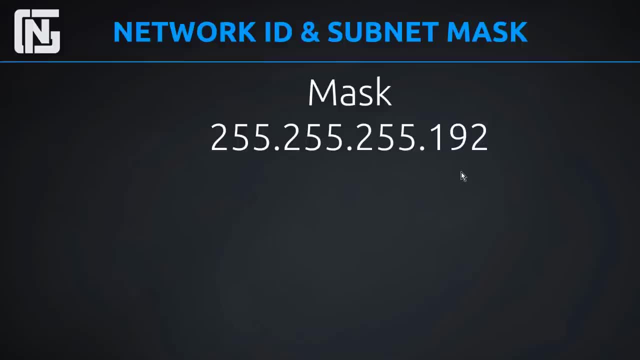 numbers in the super awesome chart. so that's just two bits in this fourth octet. so that's 8, 16, 24 and then 25, 26, so our cidr will actually be 26.. now again, we can go over this one more time. 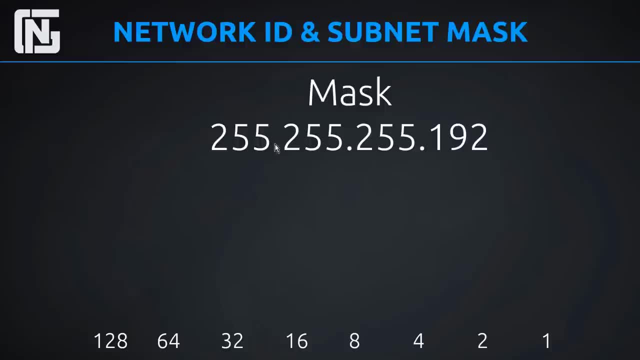 let me pull that away, and so we can find it by using our chart. so we knew all ones here, right? so this was 24. and then how many bits did we add from the last octet to to complete what we know as our cidr? one twenty four. let's say we're adding it back in our cidr format and we're adding it, so we 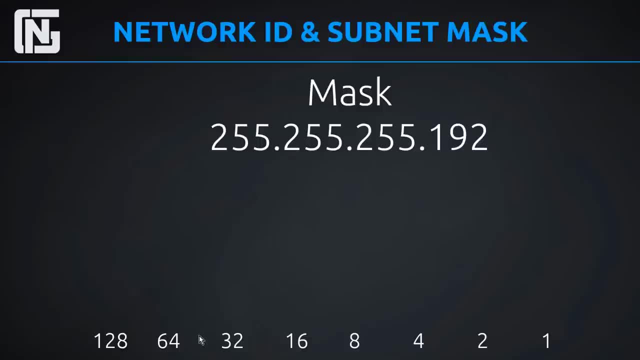 want to know how many bits make up our subnet mask. well, 128 plus 64 equals 192, and these are just two bits here, and with a subnet mask it's always going to go from left to right when you're adding it. so it's super easy to know any octet you're going to add left to right, like that for your. 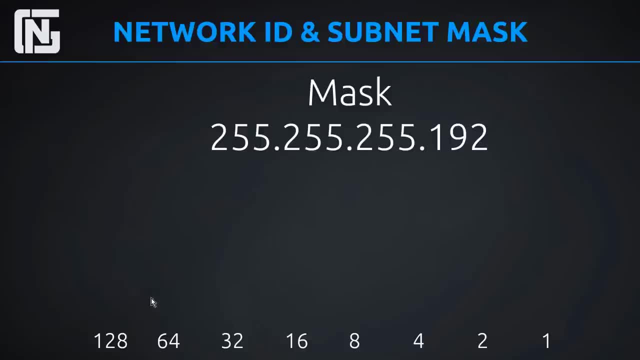 mask. so 128 plus 64 equals 192. if it was 128 plus 64 plus 32, it would be 224 in our mask right, and then 248, and then 252, and then 254 and then 255. okay, so currently we have 192 on our. 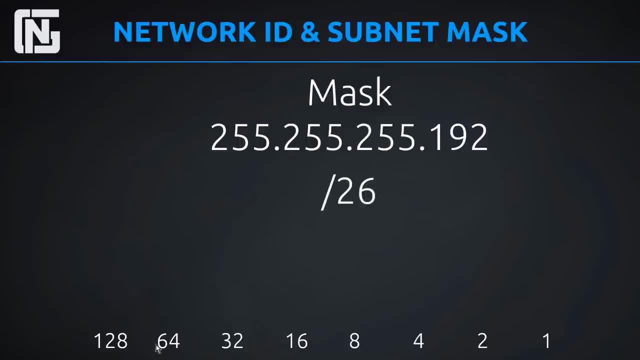 fourth octet, and we know that it's a slash 26 because these two bits here are turned on as well on our mask. now let's look at another ip address. actually it's the same ip address: 192.168.45.55. so we can look at the same ip address and, depending on what our mask is, we're. 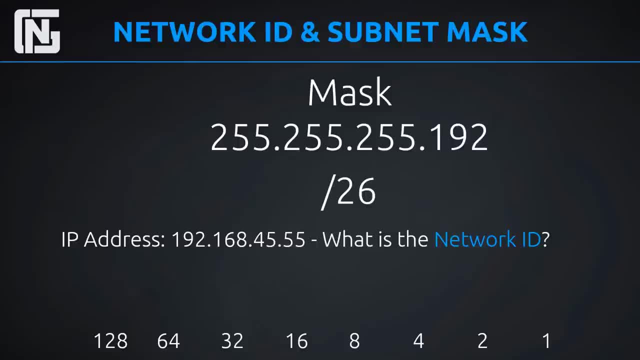 completely changing things right now. our mask was the same in the last two, so our network id stayed the same, but now we're changing it up because we have 192 there and we can go ahead and draw a box around our first three octets because we know those will not change. how do we? 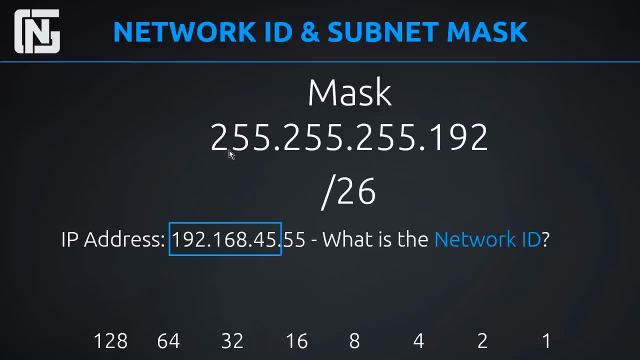 know those will not change well, because we have all 255s in the third and the first three octets, meaning that the first three octets of our ip address will be part of our network id. so our network id will start with 192.168.45. 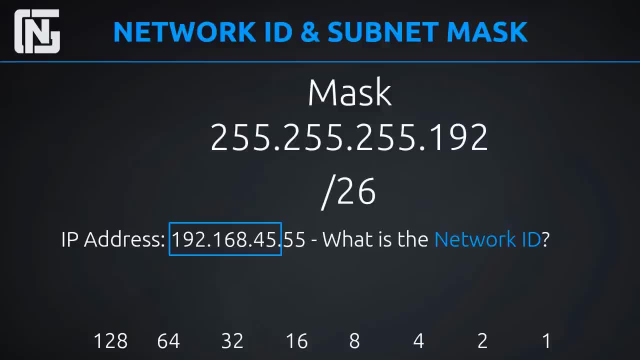 you dot something, all right. so let's figure out what that dot something is. let's look at the 55 in binary. so what is 55 in binary? that's what we get there for our fourth octet. and now we can compare this with our subnet mask which, remember, just has these first two binary bits reaching into the. 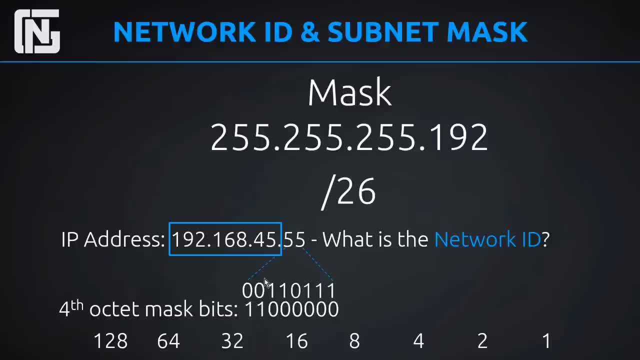 fourth octet. so the fourth octet mass bits are one one here. so we can know that everything after that is a host bit and everything before that is a subnet mask. so we can know that everything after that is a host bit and everything before that is a. 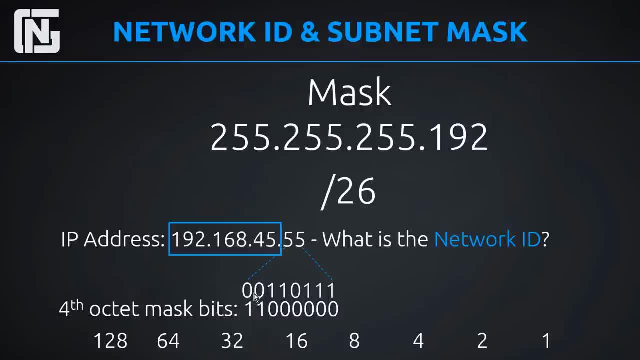 bit. Now, what is zero plus zero If we don't have 128 or 64 turned on in our IP address? well, that adds up to what guys? That adds up to zero. So our network ID is actually 192.168.45.0. 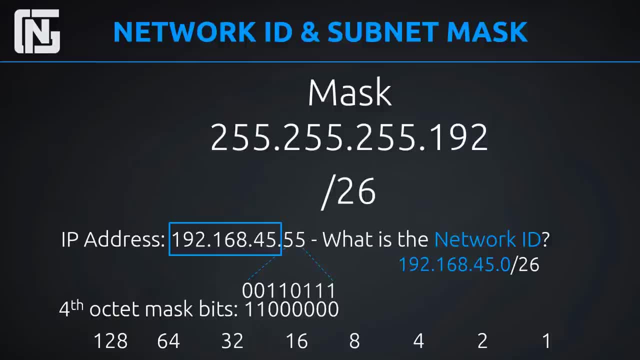 slash 26.. Now you'll also figure out, whenever we do subnetting, that this is the main work you need to do. So this is the main stuff we need to figure out, And once we write this down on a piece of paper, subnetting becomes so easy. You don't need any formulas, It's just so easy. So we'll get. 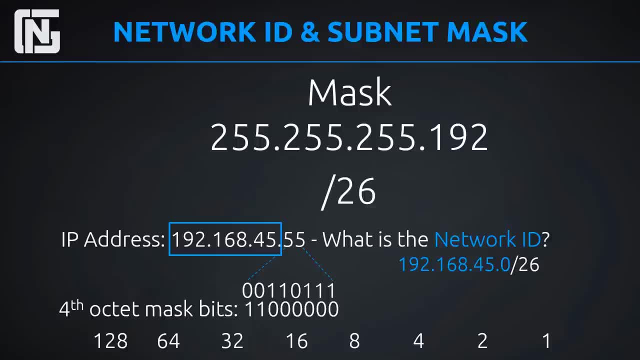 to all that later, But this is really the part you'll need to really become familiar with: converting decimal to binary, vice versa, understanding how a mask affects a network ID. Once you got that down, subnetting really is so easy. People always say subnetting is hard. 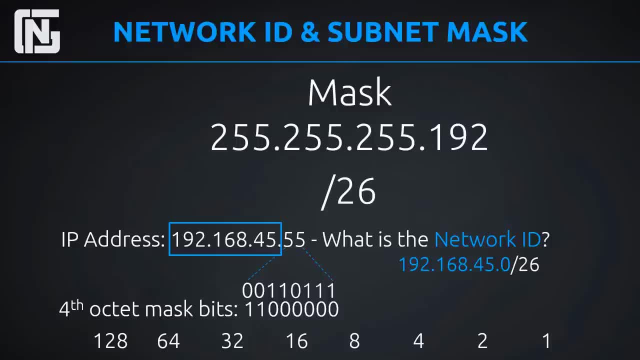 but it's not. This is what you really need to understand right here. All right, So again, our network ID is 192.168.45.0.. Now our mask does bleed into the fourth octet, But since the IP address we were given didn't have anything in these first, 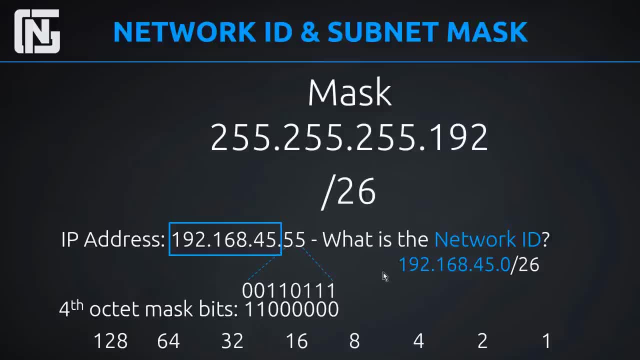 two binary digits. well, we know that this IP address is part of the 45.0 network, And so here's our mask guys, And by looking actually at this fourth octet we can say we could just actually draw a line here. So we can draw a line between our host bits and our subnetting. 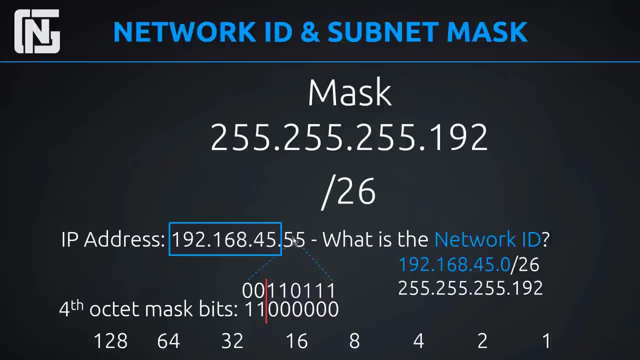 bits. Now this is useful whenever our mask goes in the middle of one of our subnetting bits. So as long as it's not, well if it's just 255.255.255.0 or 255.255.0, something like that. 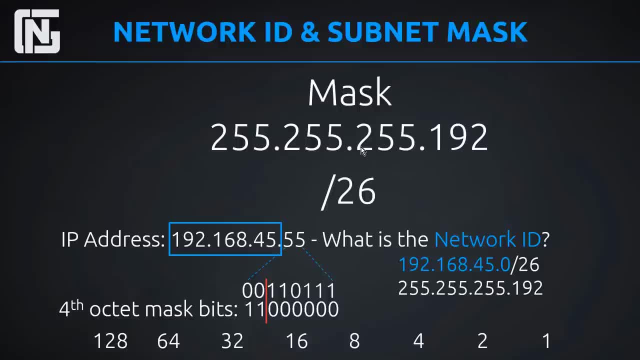 if it's just 255s and 0s, then you don't ever have to do this. But as long as it's anything else, anything other than that, it's useful to have this line. we can draw here And we can separate. 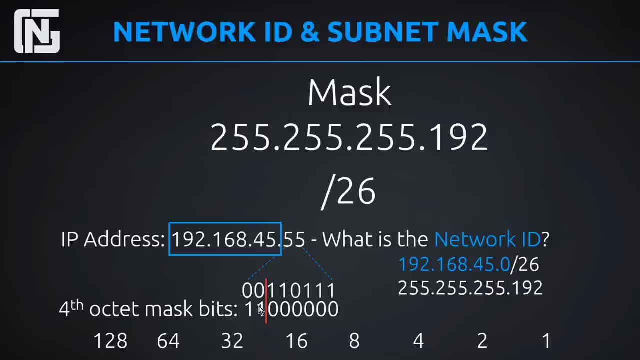 our host bits from our subnetting bits. So now we know whenever we look at our octet we can see very clearly where our subnet bits end and what's included in our subnet bits. So this is 0 and 0, which means 0 in this fourth octet for the subnet ID. So our network ID is: 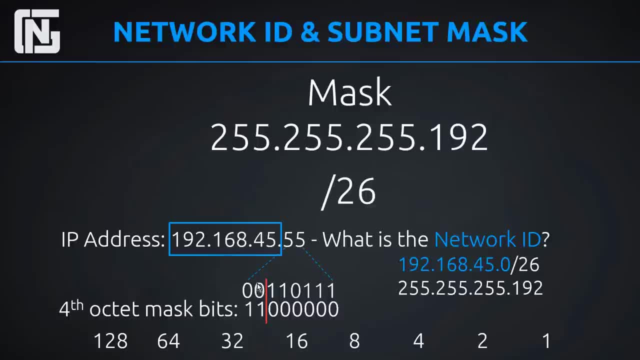 192.168.45.0.. If there was something here, if there was a 1 here, our subnet ID would actually be 192.168.45.64.. Or if there was a 1 and a 0, it would be 192.168.45.128,. actually It would. 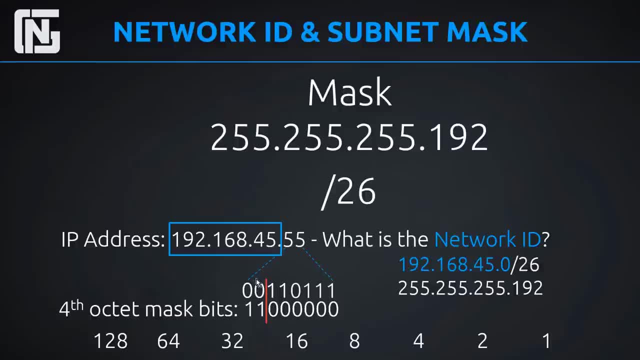 be our network ID, But in this case there's nothing there, So it's just a 0.. All right, guys, Let's move this line And we can move it down to our super awesome, cool, fantabulous, magic chart. 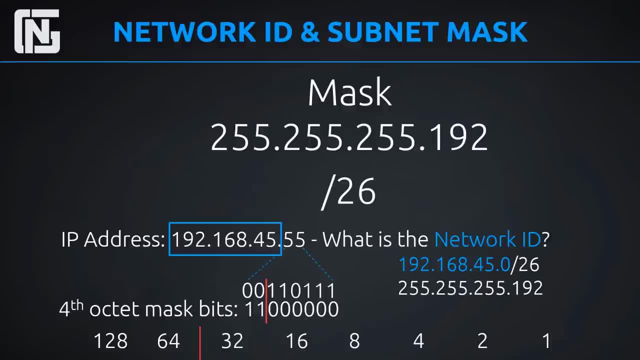 And that will also give us some great information. For example, we've moved it here past the second bit because we know that there's only two bits in the fourth octet here that we're using in our subnet mask. Now what this tells us is, if we add up all these numbers together, that will give us: 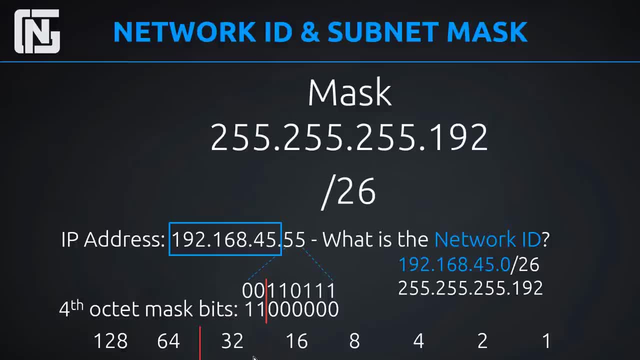 our broadcast for the network, which in this case is dot 63, right, And that's always one less than the number to the left of it. So 63 is one less than 64. So the broadcast for this network here is actually 192.168.45.63.. That will be the broadcast address If something is sent to. 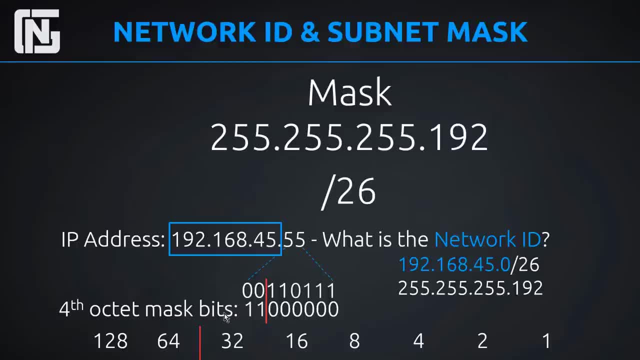 that address. it will go out to everybody on this network. It also tells us how many hosts IP address we can actually have, or how many usable IP address rather. So, if we add these all up to available addresses in this network, 62 hosts, right, Well, 62 IP addresses. Usually we're going. 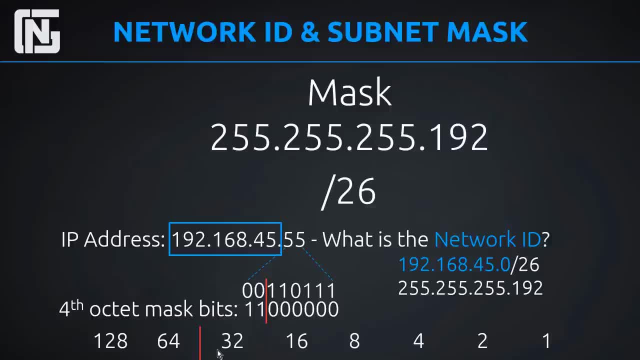 to have to assign one to our router. right, At least one to our router. So it gives us one for our router and then 61 for assigning to everybody else, But it's 62 usable IP addresses that we get from this network. All right, that's diving a little bit deep. We won't actually be doing any. 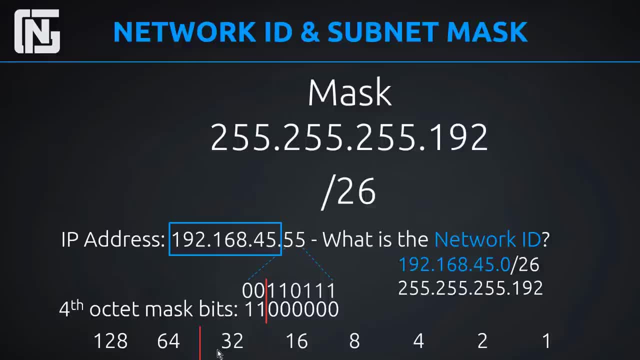 of that we just did with the line and stuff in this exercise. but that gives you a little bit of what we're going to be doing when we do subnetting and how we can make it so easy, So you don't have to worry about that. I just wanted to kind of give you an inkling of some. 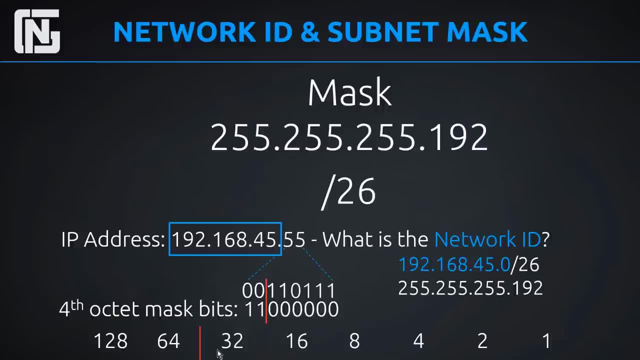 types of things you can think of and start working on if you want to, But in our practice exercises it's going to be very straightforward, So don't worry, It's going to be primarily focusing on figuring out binary to decimal conversions and then taking a subnet mask and figuring out what 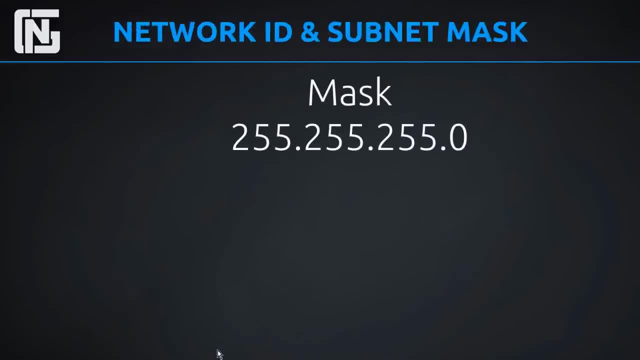 the network ID is. So let's look at another one, guys. All right, I've given you some hard ones so far, Let's do an easy one. All right, here we go. Here we have a mask: 2552552550.. And then we can say that we know what the CIDR is, because it's. 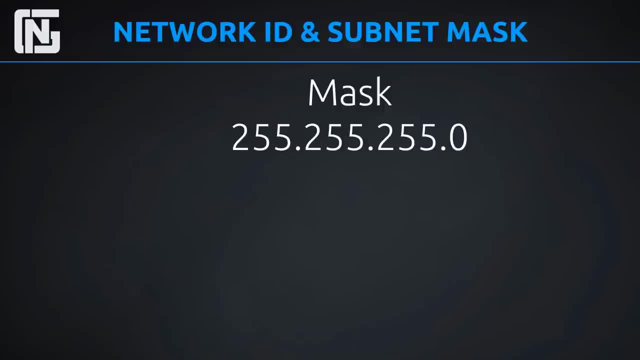 8 plus 8 plus 8.. So 8 plus 8 is 16, plus 8 is 24.. So that goes ahead and tells us- we don't have to look at our chart- that it's a slash 24 mask. This is the most common one you're going to see out. 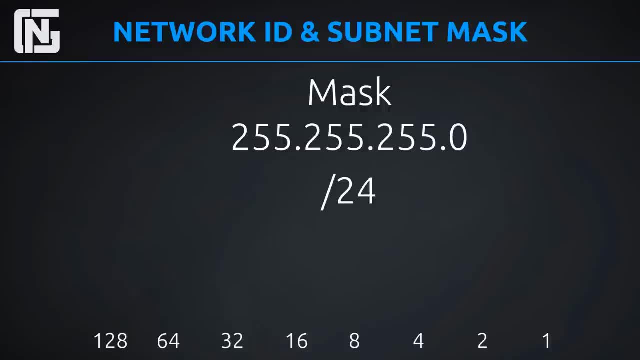 there guys, It's the most common one. It allows for 254 usable IP addresses, So that's a lot right. This is the most common one you're going to see And it's easy to write, easy to notate. 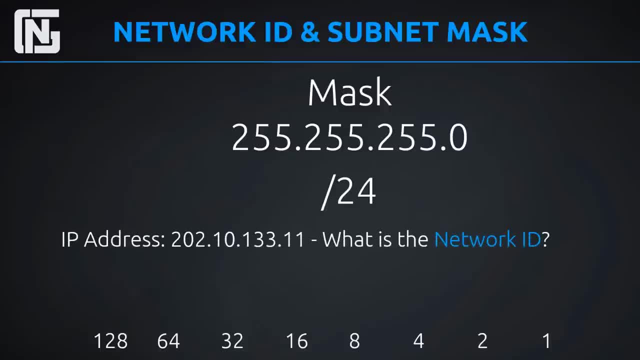 So what's the example? Well, we have this IP address here: 202.10.133.11.. What in the heck is the network ID for this IP address? What network does this IP belong to? Well, we can obviously go ahead and draw a box. 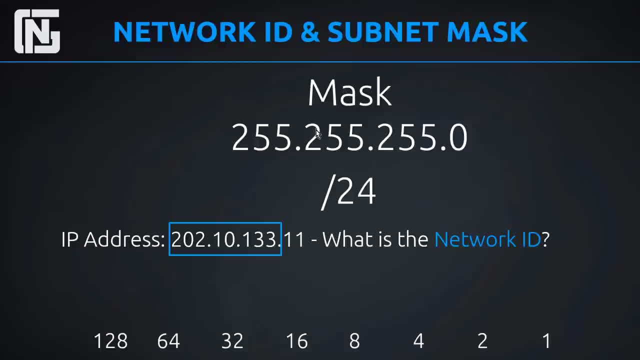 around the first three octets: 202.10.133,. right, Because we have all 255s in our mask, So we know our network ID is going to start with at least 202.10.133.. And then, well, we could break out that last octet, right? Well, we could, but guys. 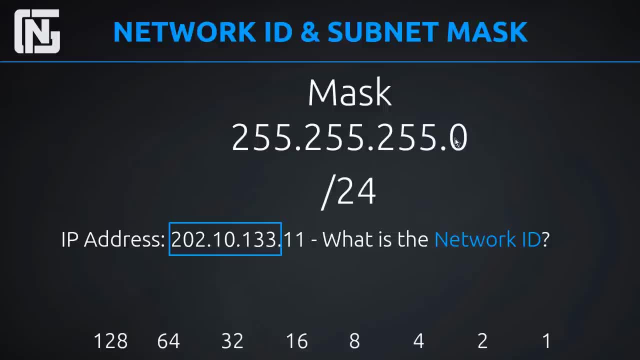 we don't need to do that at all. We actually don't need to do that because our last octet in our mask is a zero, So we don't even need to look at it. We know that our network ID is exactly what we see. 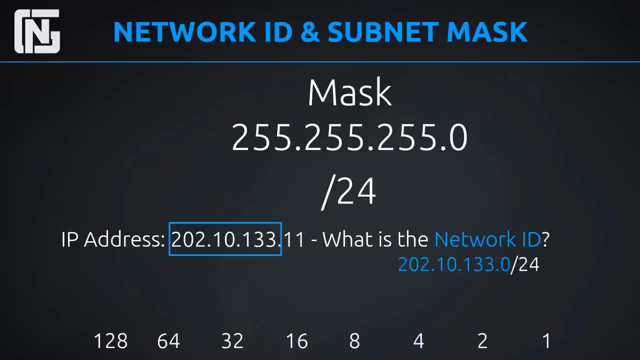 in the first three octets, and that's it. So our network ID, guys, is 202.10.133.0, with the slash 24 on the CIDR notation, And let's write the mask up there too. So that's an easy one, guys. 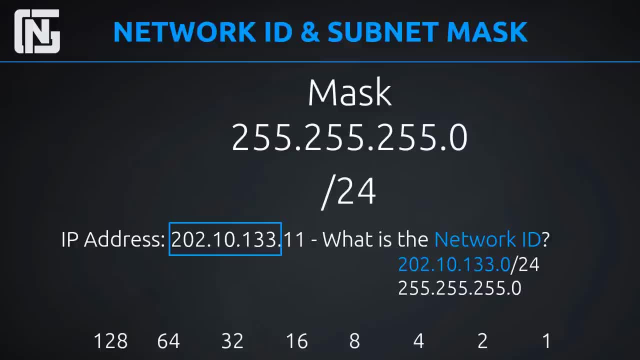 255.255.255.0.. Other easy ones are 255.00 or 255.255.00.. Those are also easy, And also 255.255.255.255.0.. That's a 32-bit mask, meaning it's exactly the IP address. You do see that out in the field.